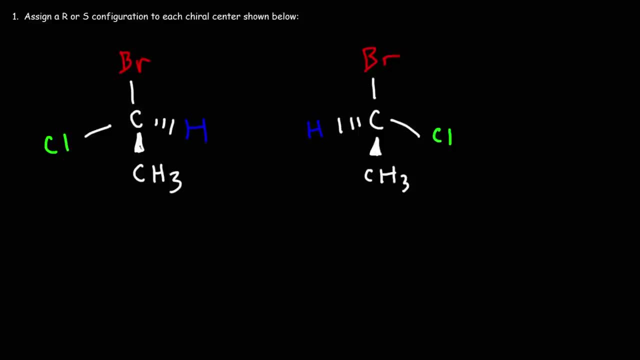 below. So first, what is a chiral center? A chiral center or a chiral carbon is a carbon atom that has four different groups attached to it. In this case, these are the four different groups. Now, in order to assign that chiral center a RS configuration, we need to rank those. 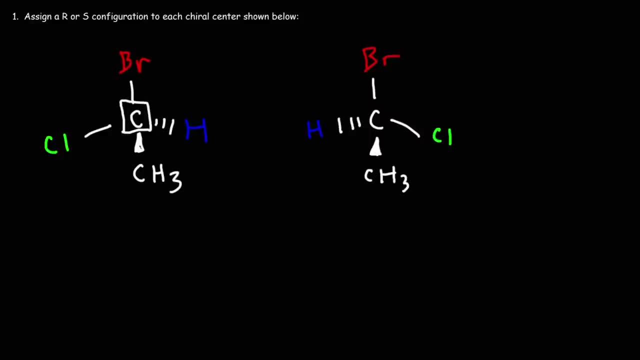 four groups using the Kahn-Ingall pre-log process. Group number one is going to have the highest priority and the way we determine priority is based on atomic number. So, looking at these four atoms- bromine, chlorine, carbon and hydrogen- which of these four atoms? 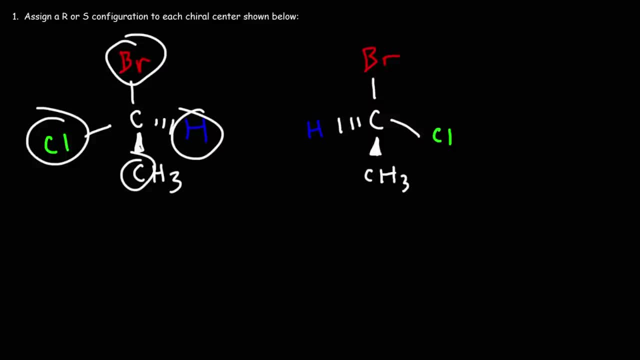 have the highest atomic number based on the periodic table. So if you're using the periodic table, you'll find that bromine has the highest atomic number. So this is going to be group number one. It has the highest priority. Chlorine has the second highest atomic number relative to bromine. so that's going to be group number two. Carbon has an atomic number of 12.. Hydrogen has the lowest atomic number of all of the elements in the periodic table. It has an atomic number of one. so it's always going to be group number four. 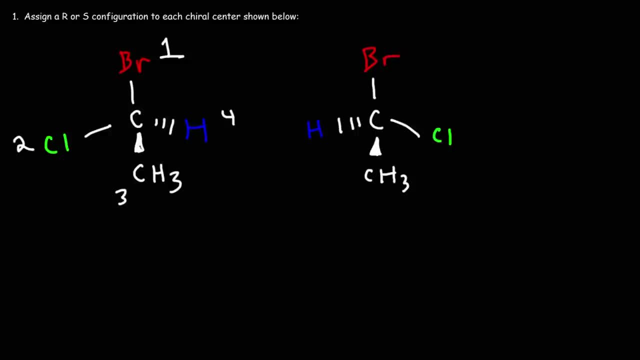 Now, before we can count it, we need to make sure group number four is in the back or it's in the hatch wedge, which it is in this case. So we can count it from one to two to three. So notice that we're rotating in the counterclockwise direction. 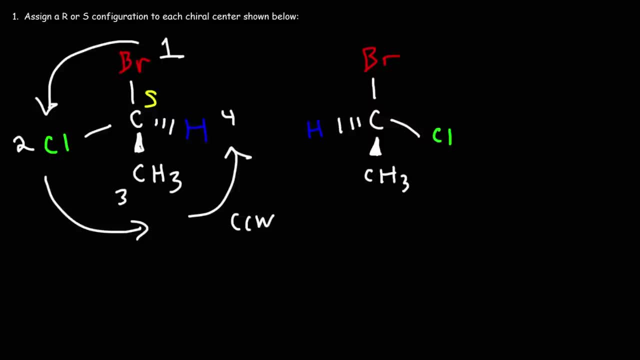 When we're rotating in the counterclockwise direction. we're rotating in the counterclockwise direction. Whenever that happens, you need to assign an S configuration if group number four is in the back. So that's the configuration for this particular chiral center. Now let's focus on the chiral center. 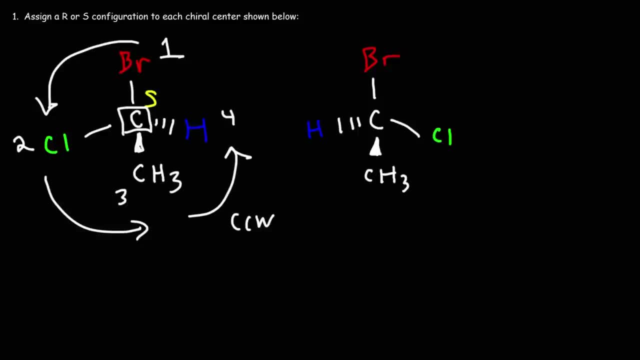 on the right and if you want to pause the video to try that example, feel free to do so. This bromine atom, we know it's going to be number one, Chlorine is going to be two, The methyl group will be group number three and H is four. So counting it from one to two to three, 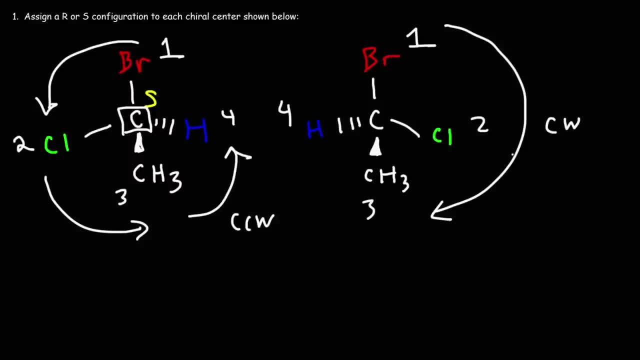 this time we are rotating in the clockwise direction, So this is going to have the R configuration. Now, looking at these two molecules, what is the relationship between them? Would you describe them as constitutional isomers, enantiomers, diastereomers, meso compounds? 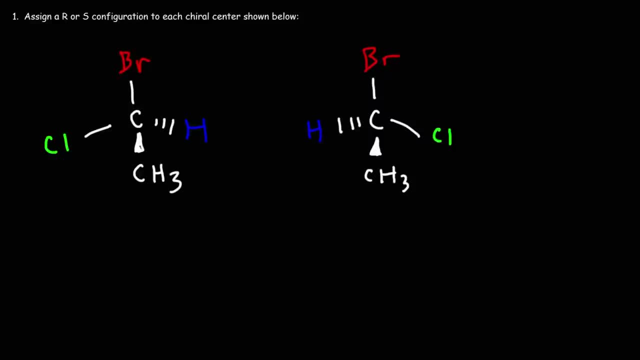 How would you describe these two compounds? Now notice that these two molecules are mirror images of each other. Therefore they are known as enantiomers. Enantiomers are a special type of stereoisomer, A stereoisomer like any other isomer. 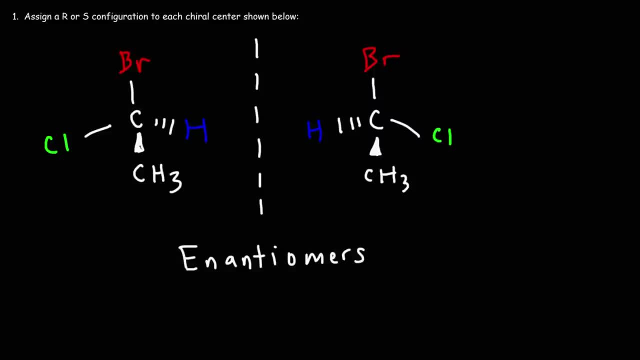 have the same chemical formula. They're connected the same way. but notice that the way the atoms are arranged in space, it's arranged in space differently. This carbon and that carbon, they're connected to the same four groups, But the way those four groups are arranged in space, they're not the same. 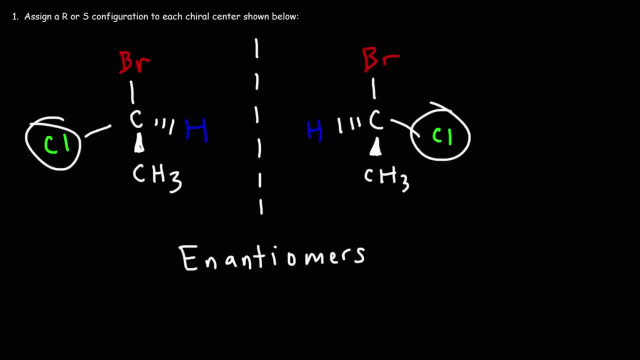 Here chlorine is on the left side, Here it's on the right side. So they are arranged in space differently, which makes it a certain type of stereoisomer. Diastereomers, enantiomers, cis-trans, geometric isomers, those are all stereoisomers, But enantiomers. 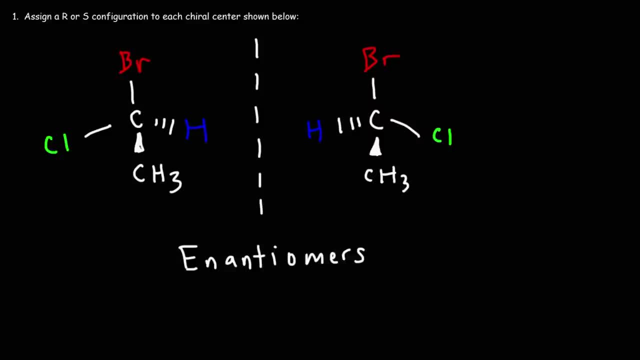 they're mirror images of each other And that's how you can distinguish them from diastereomers. Another feature of enantiomers is that they have the opposite configuration at the chiral center. Here the configuration we determine it to be S, Here 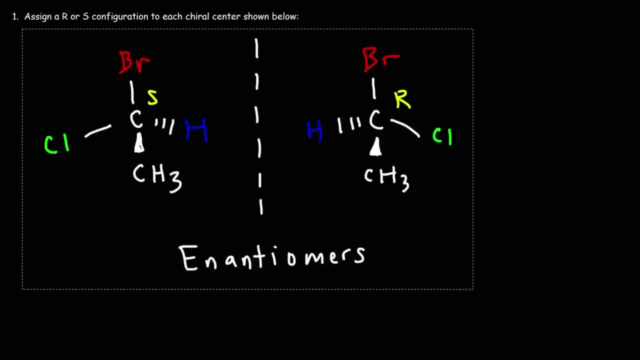 it's R. Now let's work on some more examples for the sake of practice. So go ahead and assign the R and S configuration to each chiral center that I'm going to draw. So let's put an ethyl group here. Let's add a hydrogen, a bromine atom. 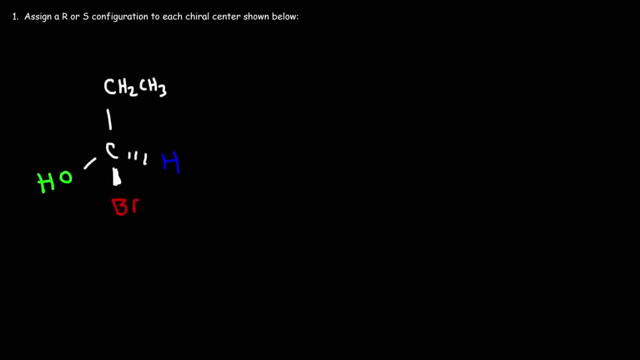 and let's put a hydroxyl group. So go ahead and determine the configuration at this carbon, And so, while you do that, I'm going to write up another one. We'll start up with a carbon with an ethyl group, And I want to make sure that my 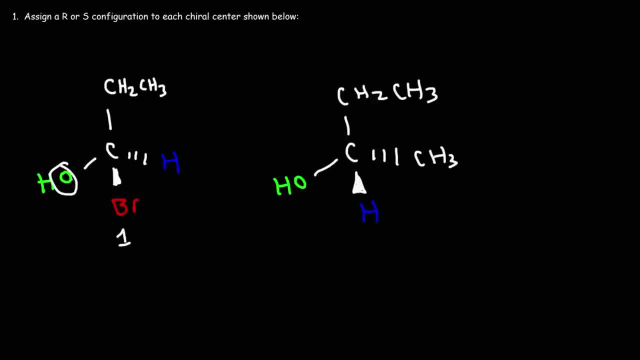 transformation is just a little bit easier with a few more alternative combinations. Another good thing about this graph will be that we'll be able to plot the differences in how closely they're going to connect. So let's start with the first one, And that's because the first thing we need to do is determine which group has the highest priority. So we know it's going to be bromine. Then, if you compare oxygen to carbon and hydrogen, we know oxygen is going to have higher priority. However, you're not only going to have more priority on a group, and you also know that the group is also going to have a higher priority. on an example, we're going to compare oxygen to carbon and hydrogen. If we compare oxygen to carbon and hydrogen, we know oxygen is going to have a higher priority. on an experiment, 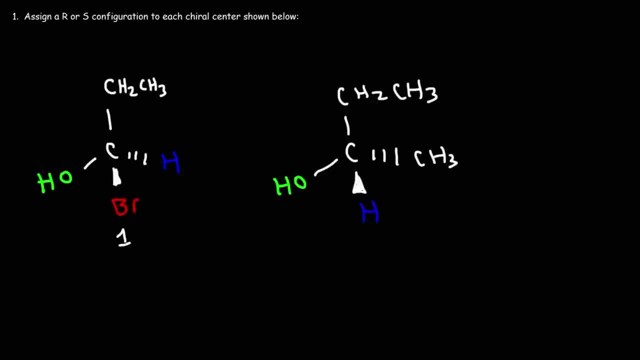 we know, oxygen is going to have a higher atomic number. The atomic number for oxygen is 8, for carbon it's 6.. So this is going to be number 2,, 3, and then hydrogen is always 4.. Now hydrogen is in the back, which is good. 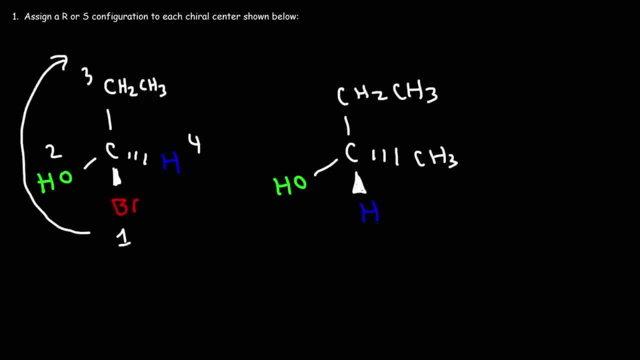 So we're going to just go from 1 to 2 to 3.. And so for this one we have the R configuration. We're rotating clockwise or in the direction of a clock. Now for the next one, hydrogen is going to be group number 4.. 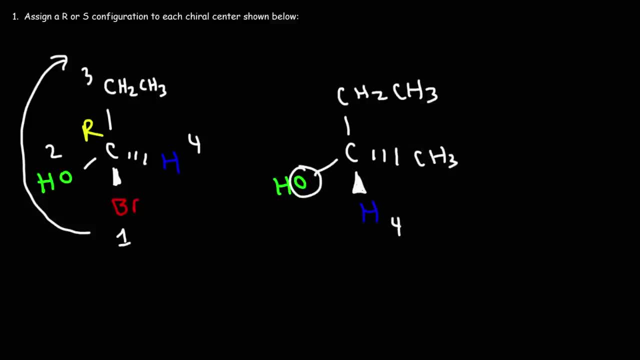 Here we have oxygen carbon, carbon Oxygen wins. so that's going to be number 1.. Next, notice that these two carbons, they have the same atomic number. So if we move on to the next group, here we have carbon versus hydrogen carbon wins. 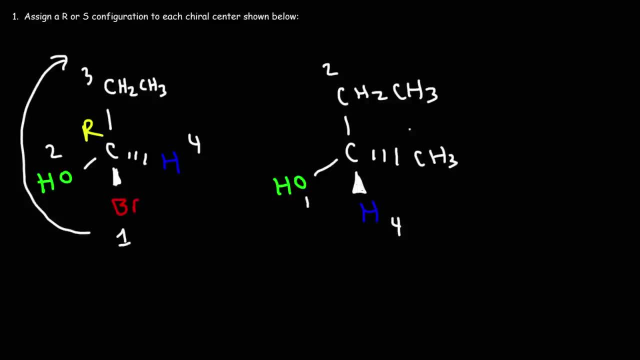 So the ethyl group has a higher priority than the methyl group. So if we count it from 1 to 2 to 3, notice that we're rotating in circles In a clockwise direction. But group number 4, it's not in the back, it's in the front. 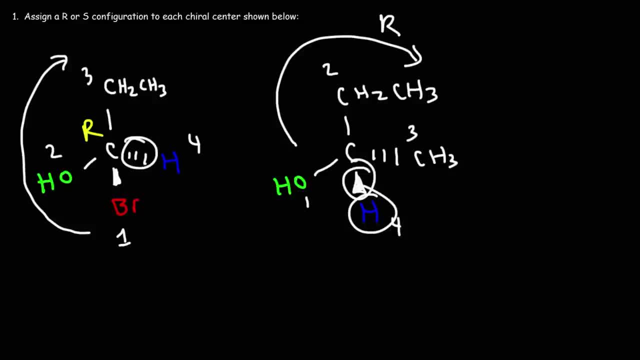 It's not on the dash this time it's on the solid wedge. So because it's on the solid wedge or it's in the front, coming out of the paper, we need to rotate it. So just switch the configuration and it's equivalent to putting group number 4 in the back. 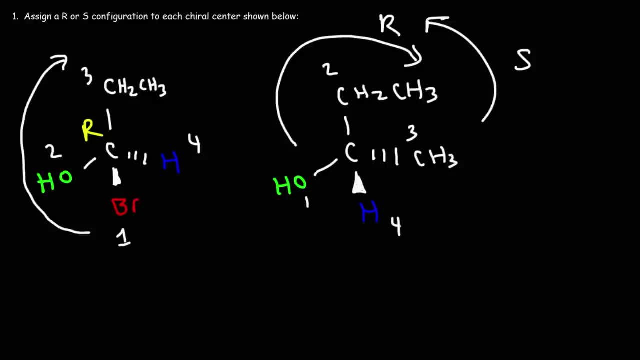 So it was R, but now it's S. So that's the configuration 4. For this chiral center. So any time H is in the front, simply count it from 1,, 2, to 3, and then reverse your answer. 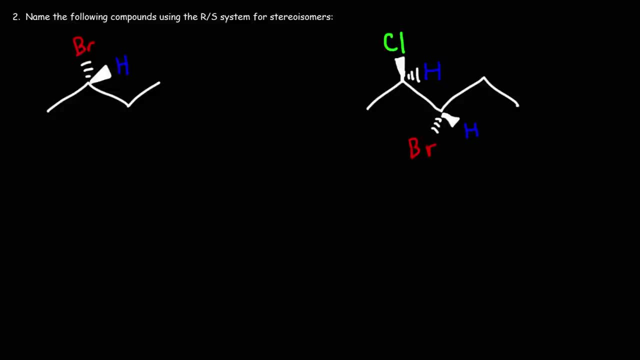 Number 2. Name the following compounds used in the RS system for stereoisomers. So first let's identify the chiral center. So let's focus on this: carbon. That carbon has a bromine, a hydrogen, a methyl group. 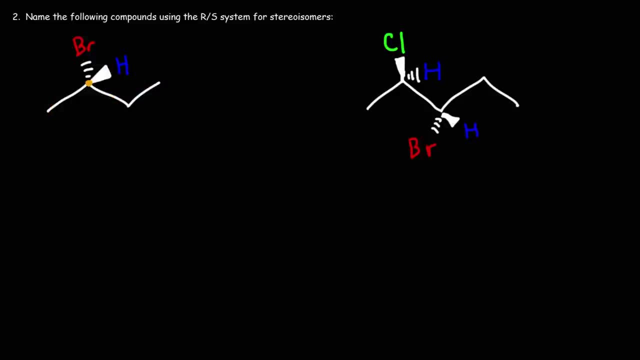 and an ethyl group. So it has 4 different groups, which makes it a chiral center. Now let's rank those groups. Bromine has the highest atomic number. that's going to be number 1.. We know ethyl has a higher priority than methyl. 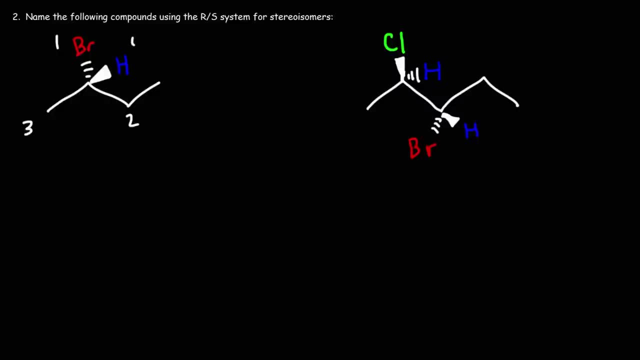 So this will be 2,, that's going to be 3.. H is going to be 4.. So, going from 1 to 2 to 3, we can see that it's going in the R direction. And when you count from 1 to 2 to 3, ignore 4.. 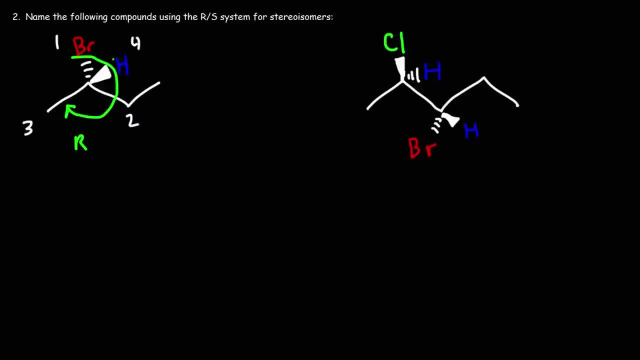 Now, after you count it, we're going to focus on 4.. 4 is a chiral center. It is in the front, It's not in the back, which means we need to reverse it. So it's going counterclockwise. 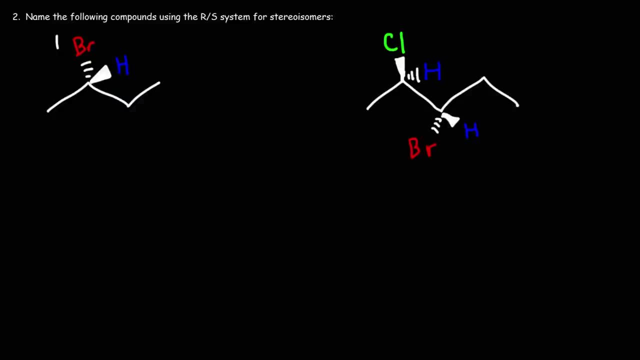 which means the configuration is S. So let's put the S configuration here. Now, in order to name it, we need to count the carbons in the parent chain. So we're going to count it in this direction. So we have a 4-carbon parent chain. 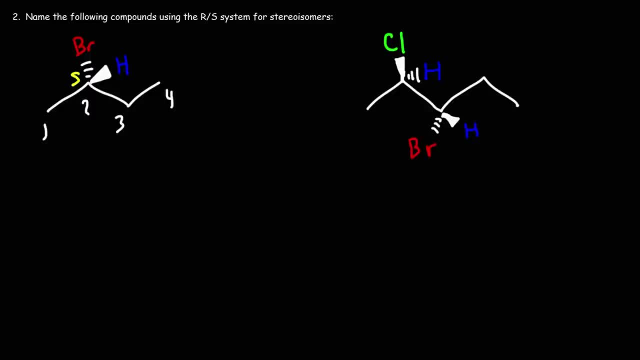 We're going to be dealing with butane. So first we need to write the configuration of the chiral center, which is S. We're going to enclose that in parentheses And then it's going to be. we have a bromine on carbon 2,. 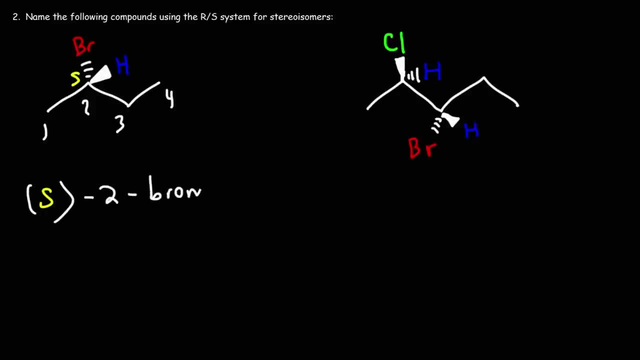 so 2-bromo. And for 4-carbon alkane, that's going to be butane, So it's S-2-bromo-butane. That's how we can name this particular stereoisomer. Now let's move on to the next one. 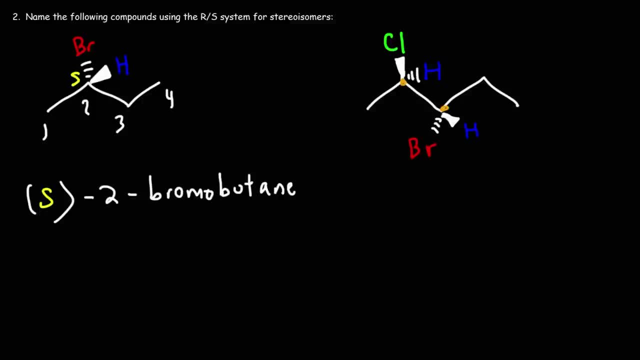 So here we have two chiral centers And you can check it. Here we have one group, two, three, Relative to this carbon. this is the fourth group If we focus on the second chiral center. this is one. group two, the ethyl-3,. 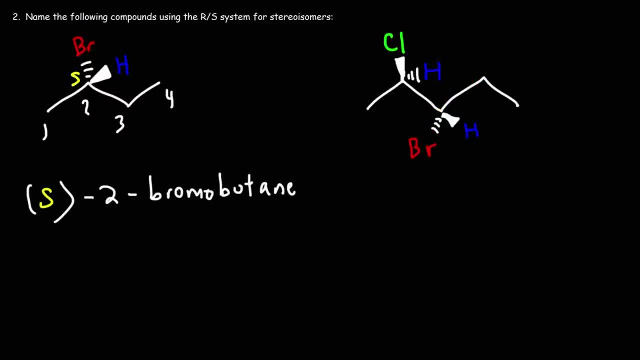 and that's the fourth group. So let's focus on the first chiral center, this one. So we're comparing a chlorine atom, hydrogen carbon carbon. So if we look at the first atom that's connected to that chiral center, 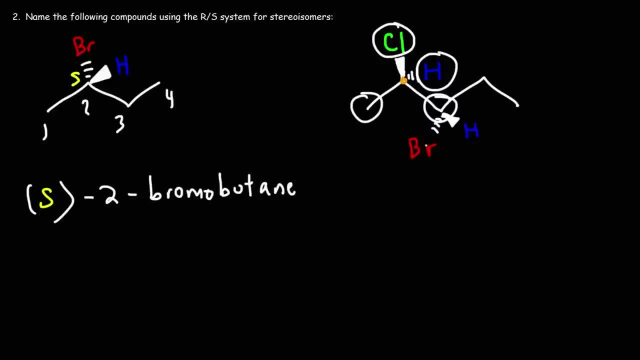 we see that chlorine has the highest atomic number. We don't look at bromine because it's not the first atom attached to this chiral center, So we look at it from a one-to-one basis. So this chlorine has a higher atomic number than that carbon. 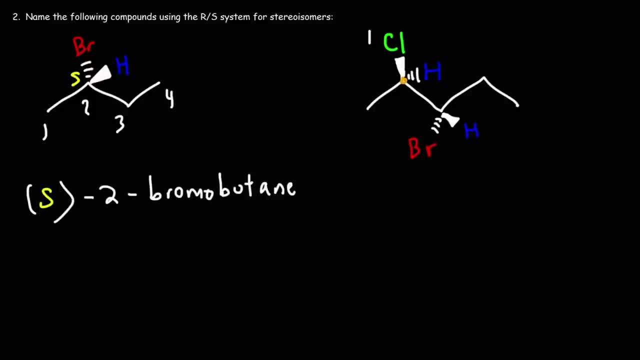 So this is going to be group number one. Now for group number two. we know H is number four, So we got to compare these two. Here we have a carbon and then a carbon, And then, after that carbon, there's a hydrogen. 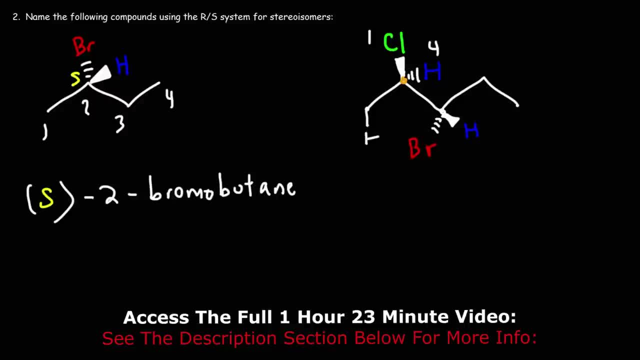 Here there's a bromine. This is going to win. So this entire group is group number three, Which makes the methyl group Actually take that back. This is two. this is number three. This has a higher priority than the methyl group. 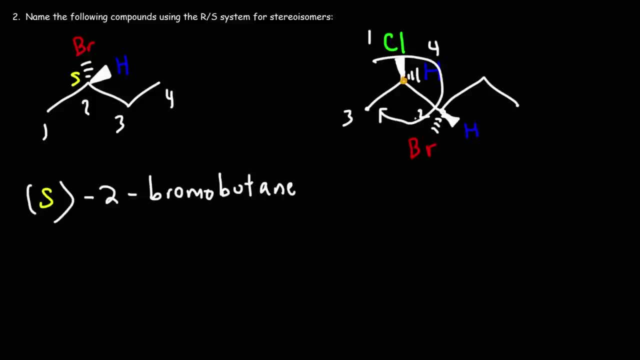 So now we can count it from one to two to three, And so that's going to be the R configuration. So let's put R here, And now let's focus on the next chiral center. So bromine, hydrogen carbon. carbon. 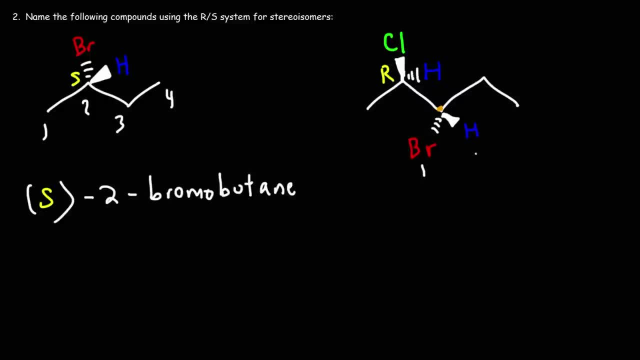 Bromine is going to have the highest atomic number, So that's one. H will be four. So now let's compare these two. So those two carbon atoms are the same. Next we have a chlorine versus a carbon. The chlorine is going to win. 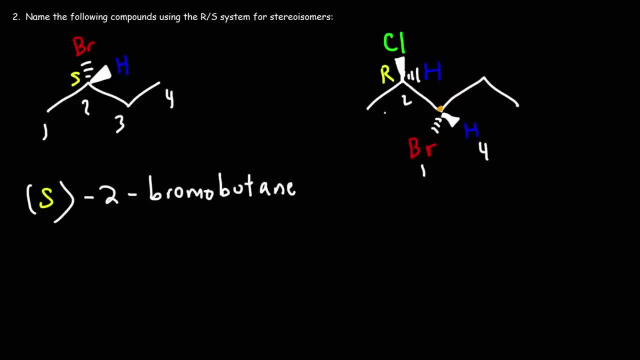 So this whole group will be group number two And the ethyl group is going to be number three. So, going from one to two to three, we're going in the R direction, But H is in the front. We're going to have to reverse it, making it S. 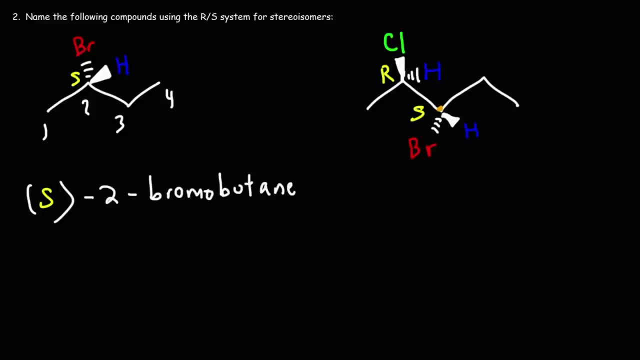 So this is S. Now that we've assigned the configuration to each chiral center, we can name this stereoisomer. So we need to number it from left to right. So the substituents will be on two, three as opposed to three, four. 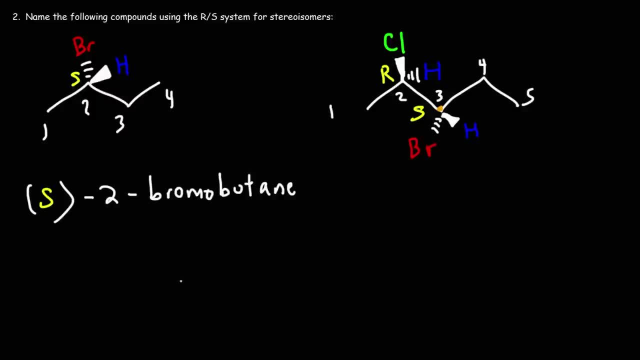 Now, on carbon two, we have the R configuration, So this is going to be two R, And on carbon three, we have the S configuration, So this is going to be three S. Now we need a comma between them, And then we need to put the bromo and the chloro group in alphabetical order. 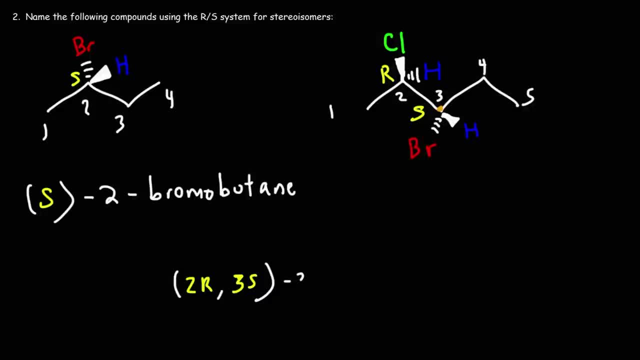 So B comes before C. This is going to be three bromo, It's on carbon three, Chlorine's on carbon two. So we're going to have two chloro And for a five carbon alkane. that's going to be pentane. 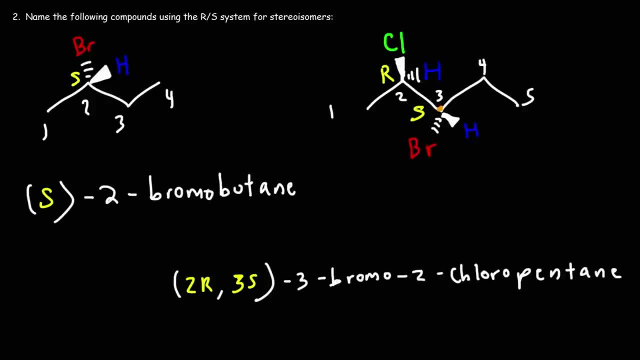 So this is two R, three S, three bromo, two chloro pentane. So that's how we can name this particular stereoisomer. Now here's a question for you: How many stereoisomers are possible if you have one chiral center? And how many are possible if you have two. So if you have one chiral center, you can have the S isomer or you can have the R isomer. So there's two possibilities. The equation that will give you the number of stereoisomers is two to the N. 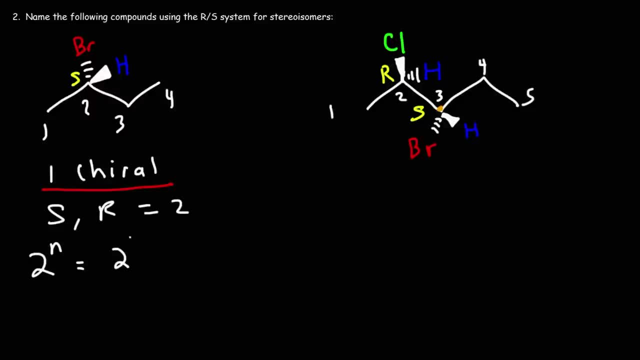 Where N is the number of chiral centers. So in this case N is one. Two to the first, power is two. So for one chiral center there are two possible stereoisomers. There are two possible stereoisomers. Now, what if we have two chiral centers? 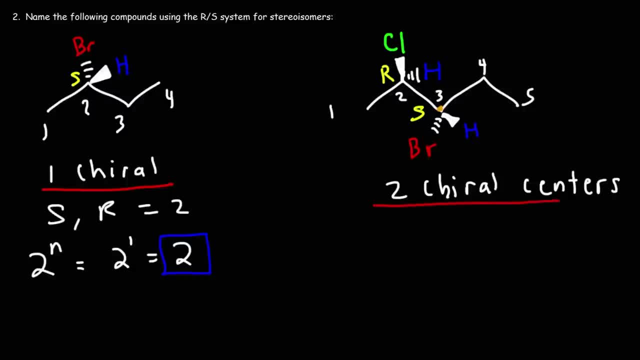 How many stereoisomers are possible? Well, it's going to be: N is two, So it's going to be two squared. Two squared is two times two, which is four. So we have four possibilities. The first possibility is if both chiral centers are R. 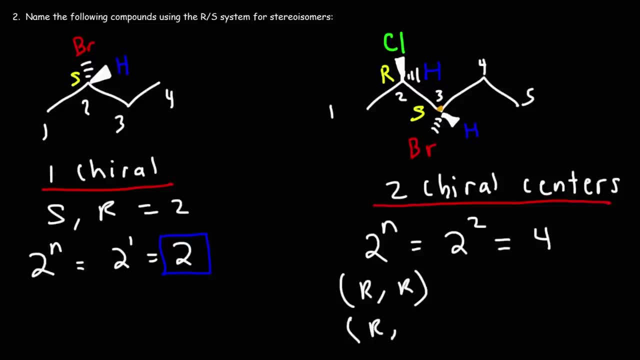 The second one is if one is R, I mean if the first one is R and the second one is S, Or if the first one is S, the second one is R, Or if they're both S. So those are the four possibilities. 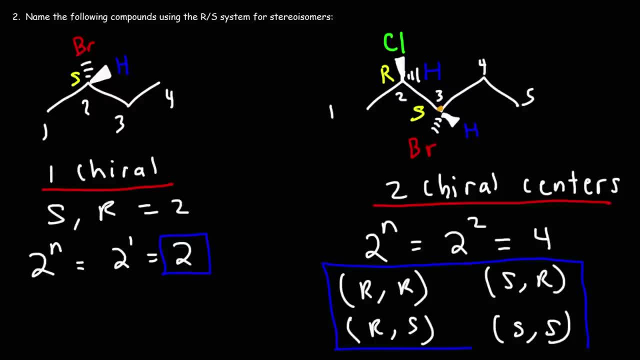 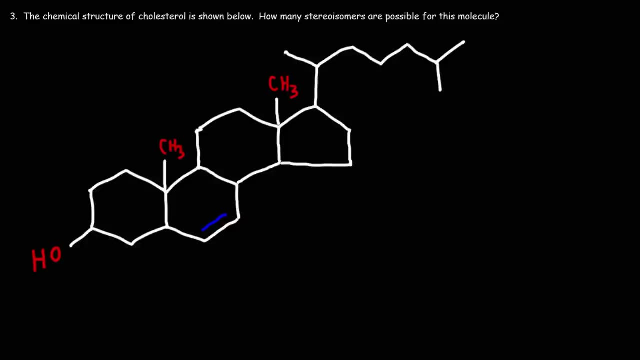 Or the four stereoisomers that are possible if you have two chiral centers. So the number of stereoisomers is going to be two to the N chiral centers. Number three: The chemical structure of cholesterol is shown below. How many stereoisomers are possible for this molecule. 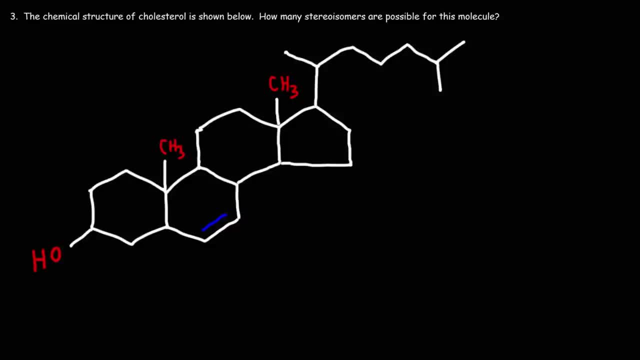 So feel free to take a minute and try this problem. So this right here is a chiral center. We have an OH group. There is an invisible hydrogen, but now it's visible. And then this side is different than that side. This side is closer to the double bond. 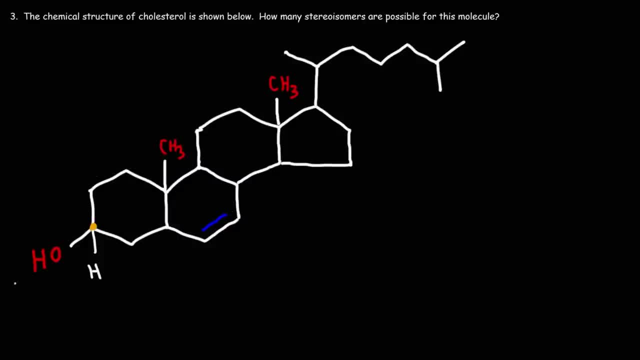 This other side has a methyl group. So these two sides are different, Which makes this a chiral center. Now, this carbon is also a chiral center. It has four different groups. Here we have a methyl group, Here is a secondary carbon. 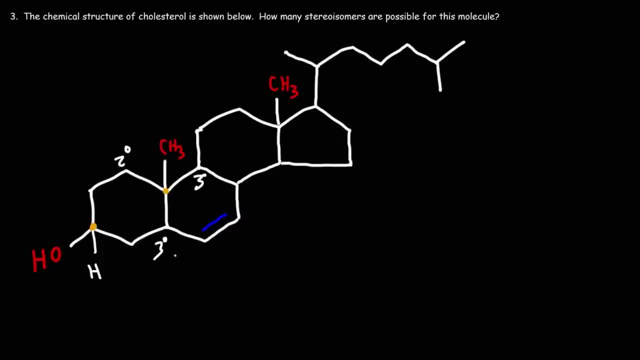 A tertiary carbon And this tertiary carbon, This tertiary carbon, is close to the double bond. This one is not, So they're different, Which makes this a chiral center. Here is another chiral center. This is one group, This is another. 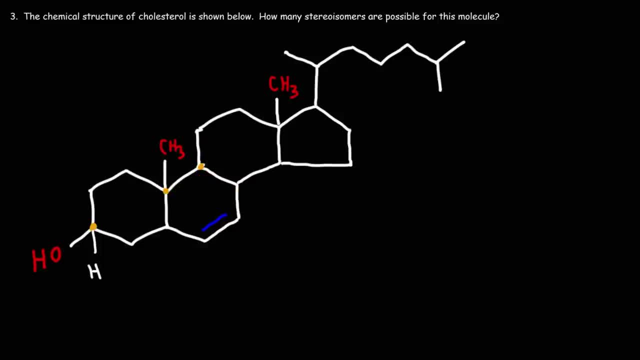 This one is another And there is a hydrogen attached to it And we could put that hydrogen here. This carbon here is not chiral. Whenever you see a carbon with two bonds and that's it. it's a CH2 carbon, Which means it doesn't have four different groups, because these are the same. 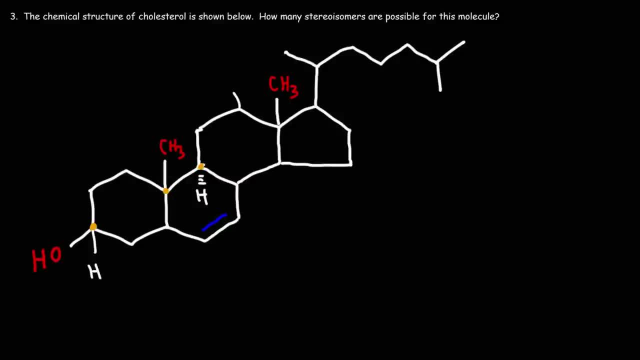 So that is not a chiral carbon. So it's best to focus on the tertiary carbons And the quaternary carbons. This is a tertiary carbon. It's attached to three other carbons And there's a hydrogen attached to it. 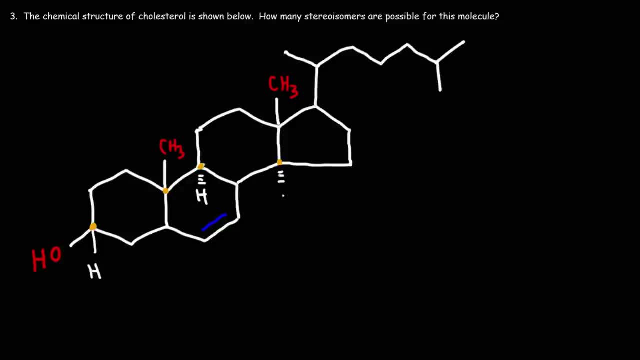 So that is another chiral center. Here's another tertiary carbon. It has three other carbons, All of which are different, And there's a hydrogen here too. Now this carbon here is quaternary. It's attached to four different carbon atoms. 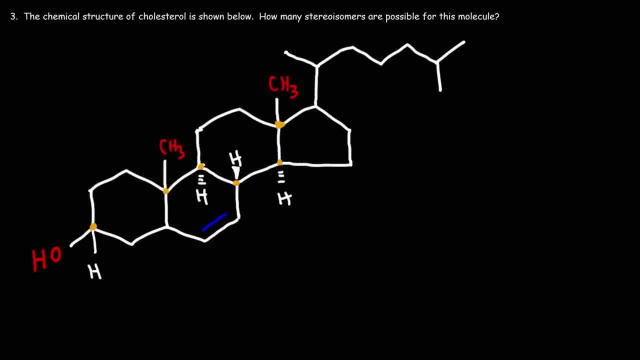 So that's another chiral carbon. This tertiary carbon is chiral 2.. There's a hydrogen here And this carbon is tertiary And it's chiral. This is group 1.. This is another group. This is another group. 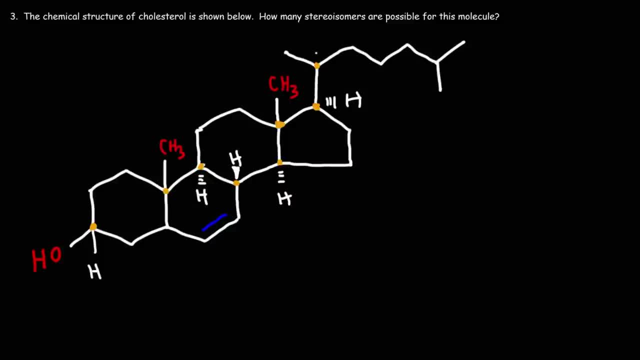 And then the hydrogen is the fourth group. The hydrogen is the fourth group, So let's put that hydrogen on the hatch wedge Now. this carbon here is tertiary, but it's not chiral Because it doesn't have four different groups. These two methyl groups are the same. 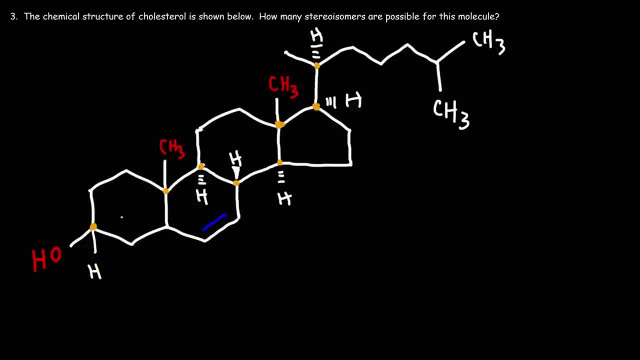 Thus cholesterol has a total of one, two, three, four, five, six, seven, eight chiral centers. So because cholesterol has eight chiral centers, it's going to have two to the eight stereoisomers. Two to the eight is two to the four times two to the four. 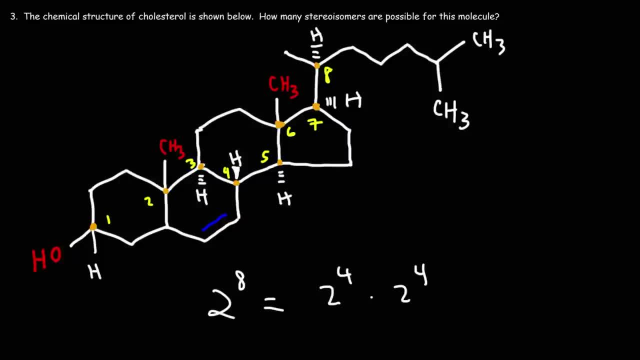 Four plus four is eight. If you multiply two, four times two times two is four times two is eight times two is sixteen. you get sixteen times sixteen, which is two hundred and fifty-six. So this is the number of stereoisomers. 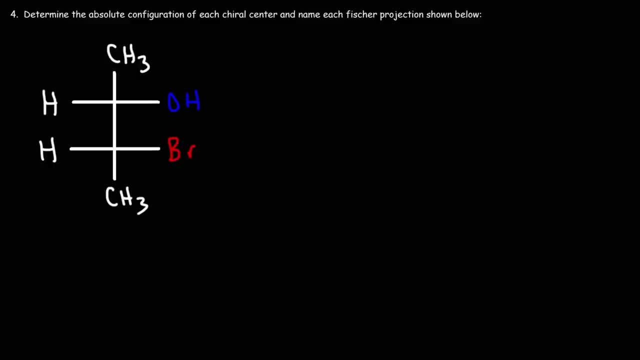 that are possible for this particular molecule. Number four: Determine the absolute configuration of each chiral center and name each Fischer projection shown below. When dealing with Fischer projections it's easy to determine the chiral center. So we have two chiral centers, which means that we have: 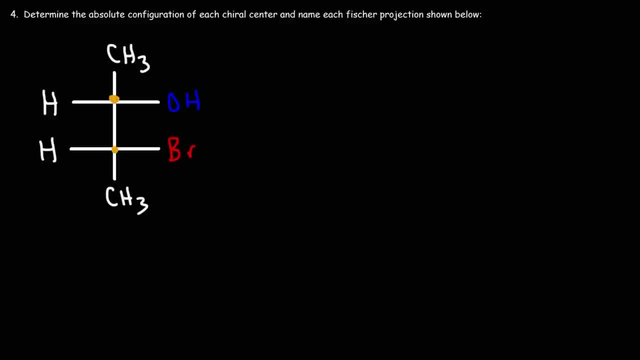 four possible stereoisomers for this particular structure. Now, before we determine the absolute configuration of each chiral center, let's talk about Fischer projections. So let's say, if we have this particular Fischer projection, Let's make this an ethyl group. 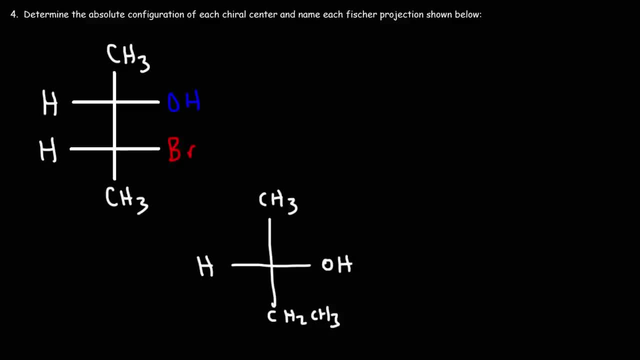 And let's say: this is hydrogen, this is OH. What we need to realize is that the groups on the horizontal part of the Fischer projection, they're in the front, So you can redraw the structure like this if you want. They're coming out of the page. 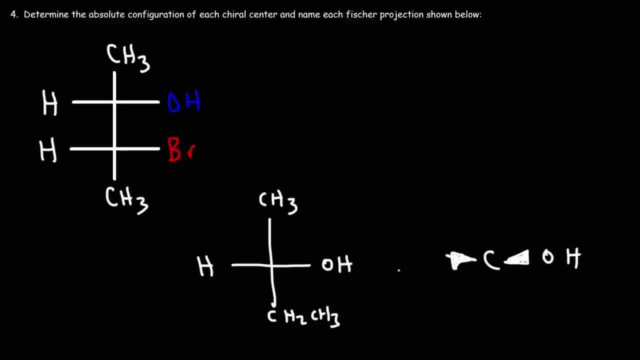 And so they're on the solid wedge, These two groups. they're on the dash or the hatch wedge, So they're going into the page. You can view them as being in the back, So make sure you understand that. Now, hydrogen is typically on the side. 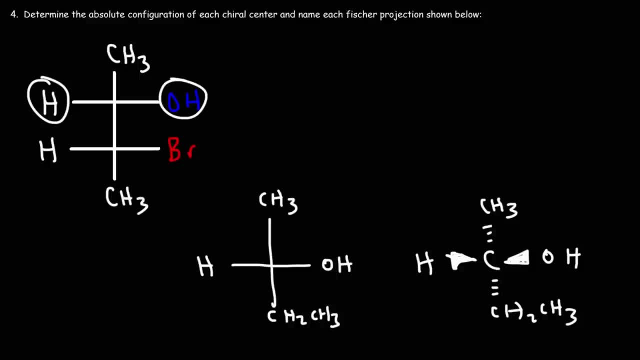 which means that, as group number four, you're going to have to reverse it when determining the configuration. So keep that in mind. Any time group number four is in the front, you need to reverse it. So let's begin by determining the configuration of this chiral center. 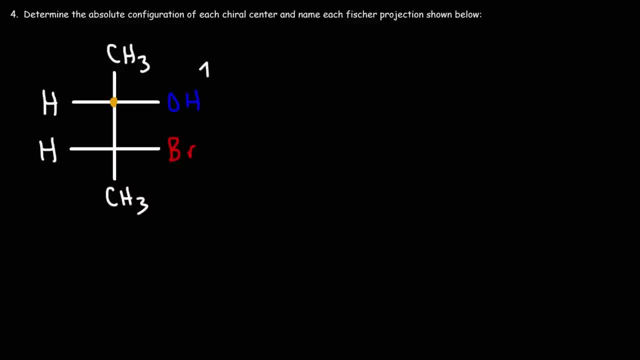 The hydroxyl group is going to be group number one. Oxygen beats these two carbon atoms. Now, comparing those two carbon atoms, they're the same, But here we have a bromine, Here is a hydrogen. So this group has a higher priority than the methyl group. 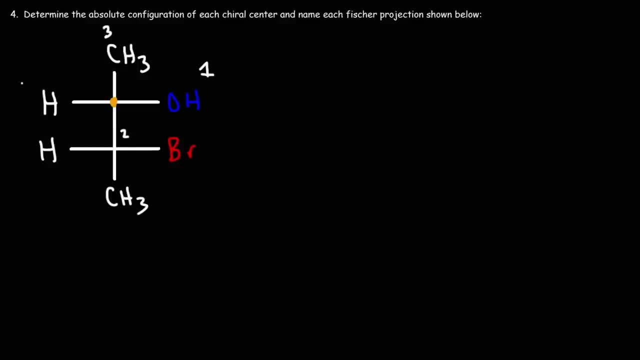 So this will be group number two, The methyl will be three And then hydrogen is always four If it's there. So going from one to two to three, we're going in a clockwise direction. So that's R, But H, remember H. 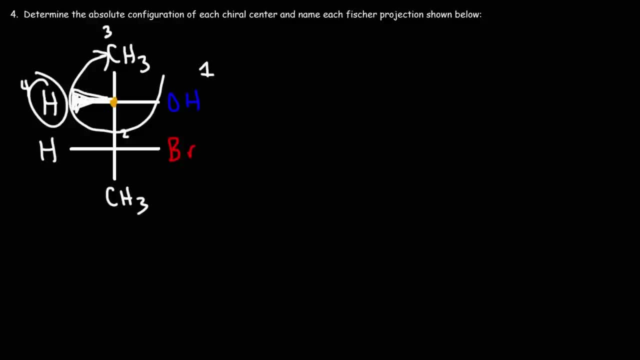 when it's in a horizontal part, it's like being on the solid wedge. H is in the front, So we got to reverse it. So we're going to get S. So we have the S configuration for that chiral center. Now for the next one. 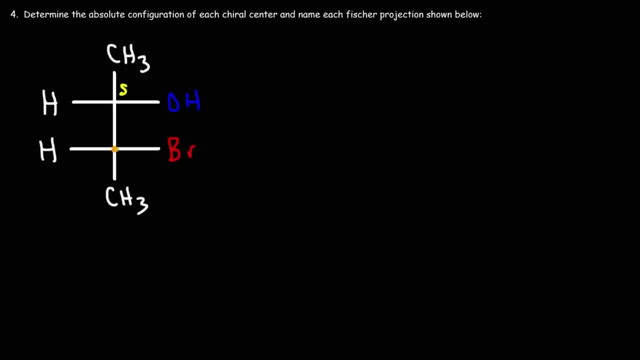 So we're going to focus on this. chiral center. Bromine is going to be group number one. It has the highest priority. Next, we're comparing the methyl group with this group, So we have carbon to carbon And then hydrogen to oxygen. 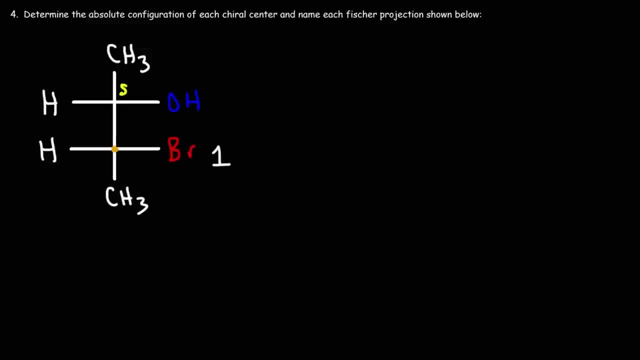 Oxygen wins. So this entire group is going to be number two. Methyl is three, H is four. So, going from one to two to three, it looks like we're going in the S direction, But if we reverse it it's going to be R. 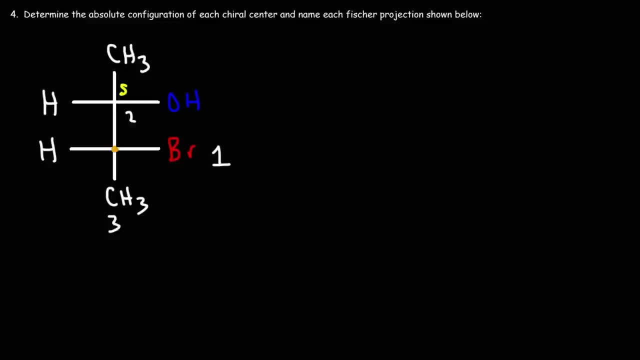 So we have the R configuration here. So now that we've assigned the absolute configuration to each chiral center, we can go ahead and name this particular molecule. So the hydroxyl group is going to have priority over the bromine group. So we're going to count it in a way that. 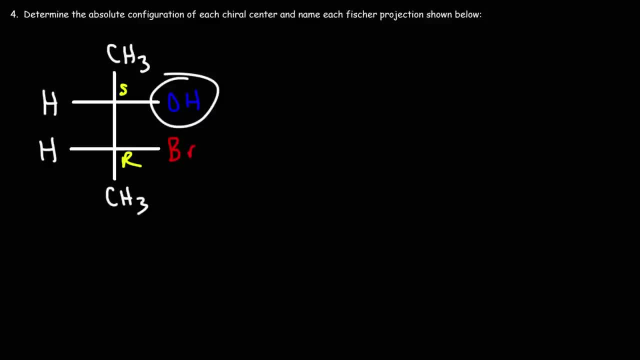 we give the hydroxyl group the lower number. We want to give it a two instead of a three, So we're going to count it in this direction. So, on carbon two, we have the S configuration, So this is going to be 2S. 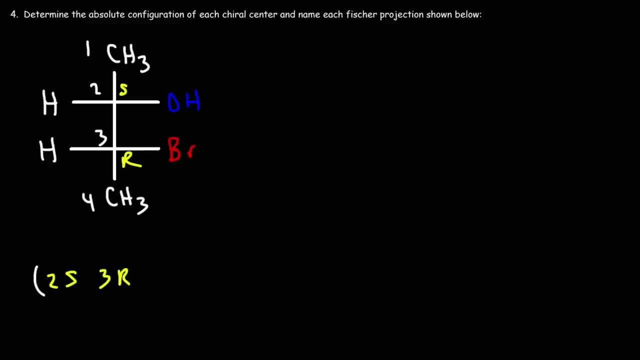 And on carbon three we have the R configuration, So 3R, And then we have a bromine on carbon three, So this is going to be 3-bromo And the alcohol is going to be part of the parent name. 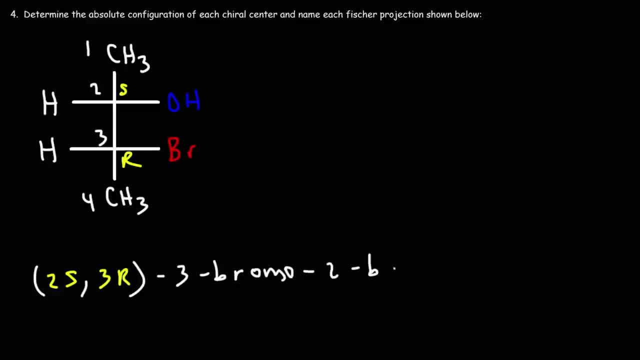 And it's on carbon two, So it's going to be 2-butanol, because we have a four-carbon chain. So 2S, 3R, 3-bromo 2-butanol- That's how we can name this particular fissure projection. 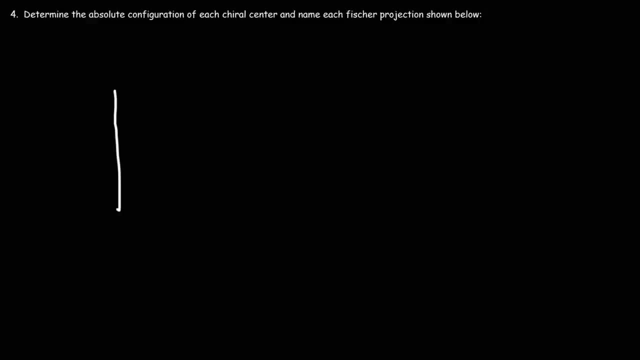 Now let's try another example. Go ahead and name this fissure projection and determine the configuration at each chiral center, just like we did before. So let's start with this one. Bromine is going to be group number one, This group with the chlorine atom. 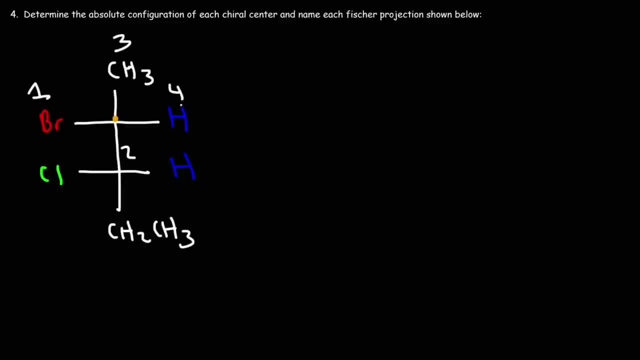 we know that's going to be two. Methyl is three, H is four. So going from one to two to three, ignoring four, this is going in the counterclockwise direction. So that's S, But H is in the front, so we need to reverse it. 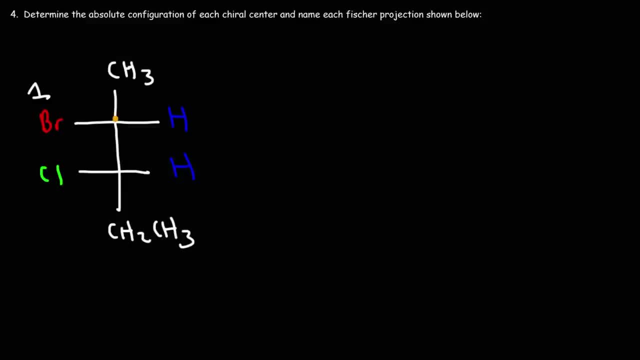 So we're going to get R for the first one. Now for the second chiral center, chlorine is going to be group number one. This entire group is number two. If we compare carbon to carbon, it's a tie. And then carbon to bromine: bromine wins. 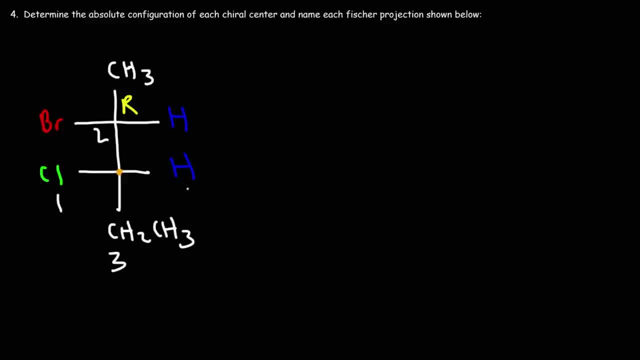 So this is number two, Ethyl is number three, H is four, So going from one to two to three, skipping four. it appears to be R, But H is in the front, so we reverse it And we get the S configuration. 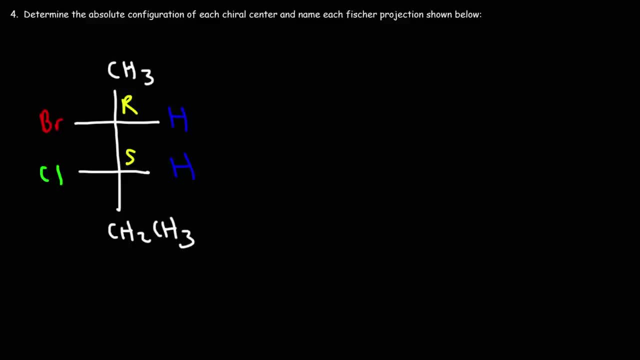 So now that we have the configuration at both chiral centers, we can name it. So we don't want to count in this direction, because this will be three and that will be four. Rather, we want to count in this direction. So this will be two and this will be three. 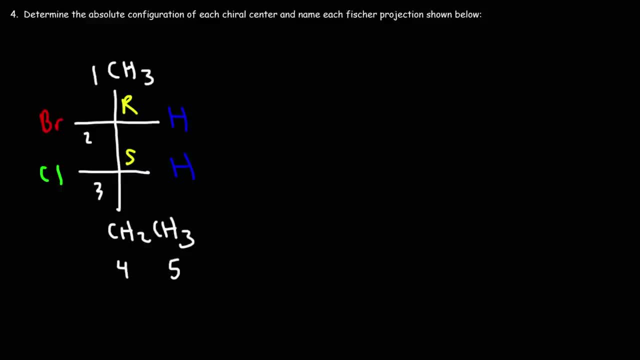 So we have a five carbon chain. so we're dealing with pentane. But first let's focus on the configuration. So the configuration is R at carbon two, So we're going to have two R And then it's S at carbon three. 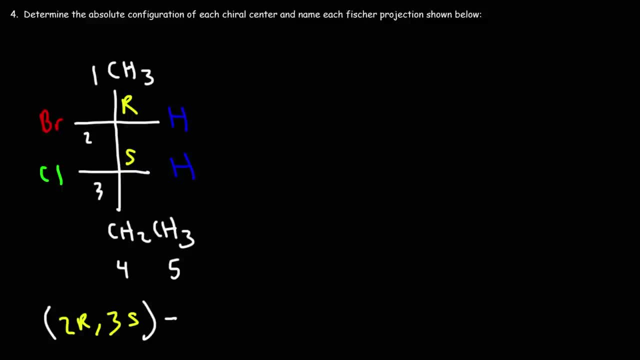 So three S. And then we have a Br on carbon two, And we need to put it in alphabetical order- B comes before C, So this is going to be two bromo. And then we have a Cl on carbon three, So three chloro. 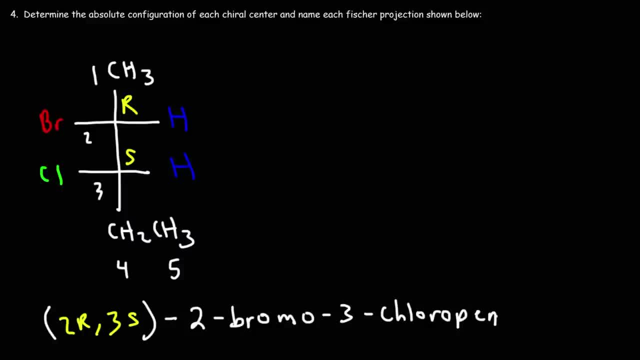 And then for the five carbon chain that's going to be pentane. So that's the nomenclature or the IUPAC nomenclature for this particular fissure projection. It's two R, three S, two bromo, three chloro pentane. 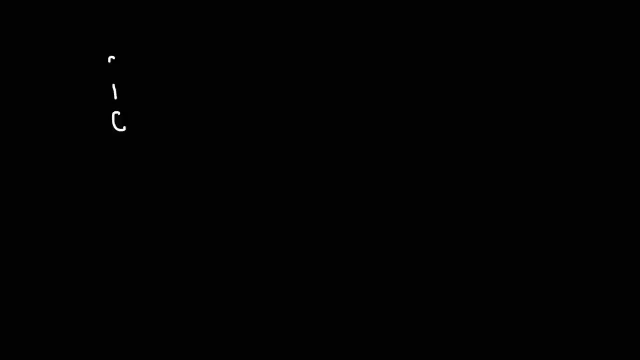 Now let's work on a more challenging problem. So let's say, this chiral center has an ethyl group, a methyl group in the front And let's put a chlorine group in the back And a hydrogen. Go ahead and assign the configuration to the chiral carbon. 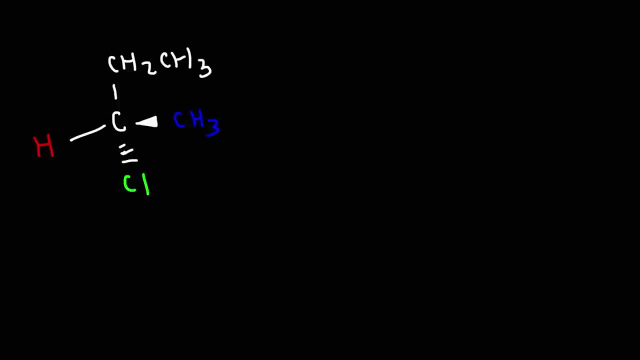 Is it R or S? Now this problem is different, because hydrogen group number four is neither in the front nor is it in the back. So how do you assign the configuration in this situation? Well, let's begin. We know that chlorine has the highest atomic number. 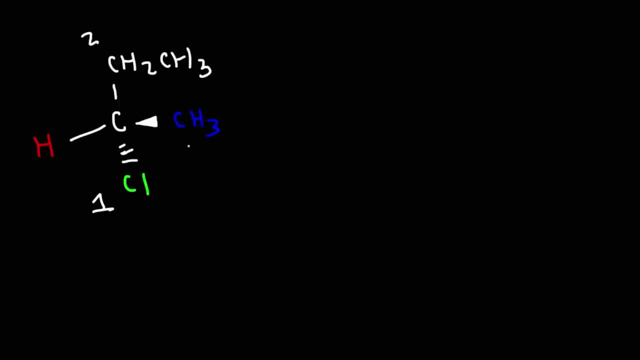 so that's going to be group number one. Ethyl has more priority than methyl, so ethyl is two, methyl is three, H is four. In a situation like this, there's a technique that you could use to assign the configuration. 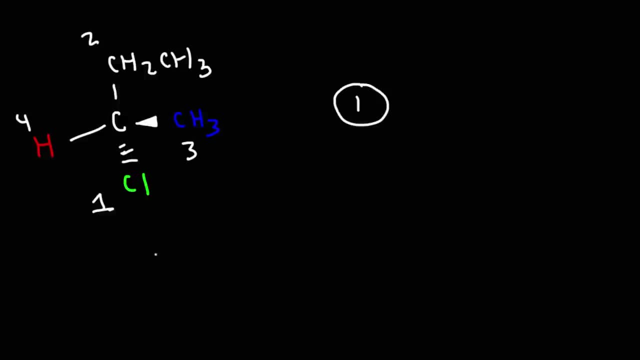 Whatever group is in the back, put it in a circle. So I'm going to put one in the circle And you could put a small subscript B to indicate that whatever's in the circle is in the back. Sometimes it could be in the front. 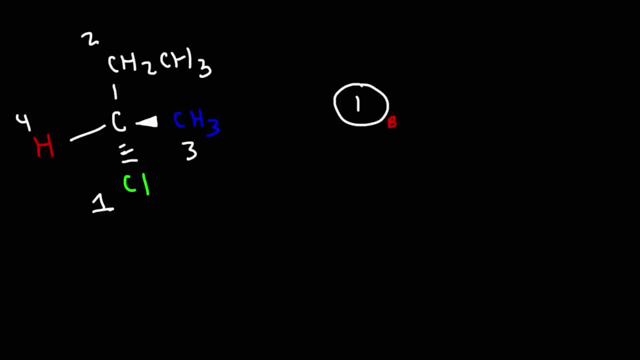 But for now, whatever's in the circle in this problem is in the back. Now the other numbers: two, four and three. you want to arrange them in the form of a triangle. Now, if you notice, two is at the top, so let's put that at the top. 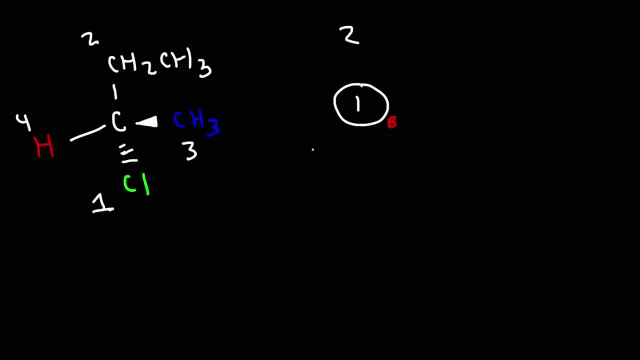 Four is at the bottom left with respect to two, so let's put that here. Three is on the bottom right. Now what we're going to do is we're going to rotate this molecule in such a way that number four will be at the top where two is. 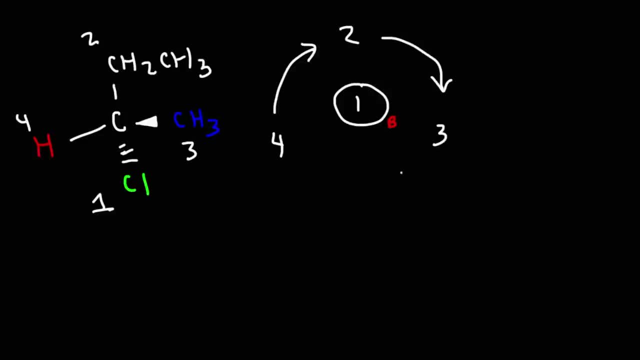 So we're going to rotate it 120 degrees clockwise. So one is still in the circle. Four has replaced two. Two is now where three was And three is where four was. Now the next thing we're going to do is we're going to flip the molecule. 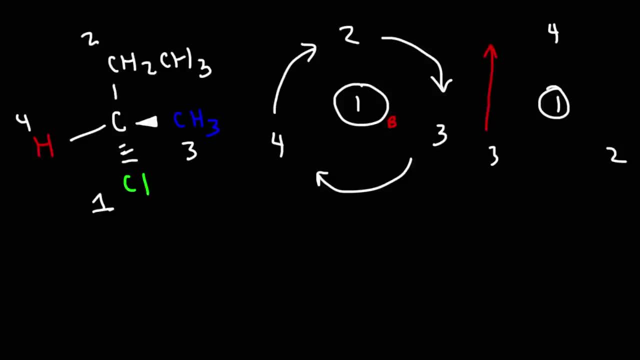 As we flip it, two and three will move to the top. Group number four is going to expel group number one, So now four is in the circle, one is beneath it, and then three and two are at the top, Now four. 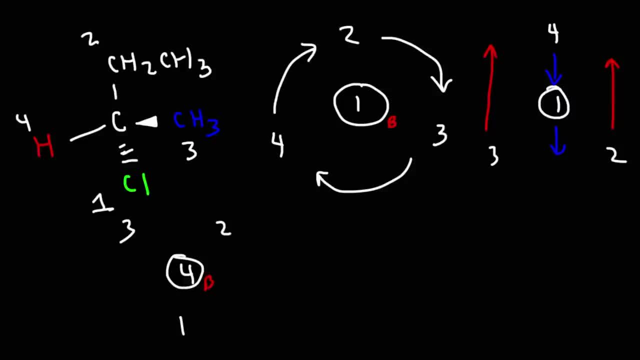 group number four is in the back, because what's in the circle represents what's in the back, And so we can count it from one to two to three, and this gives us the S isomer. So the configuration at this Carroll Center is S. 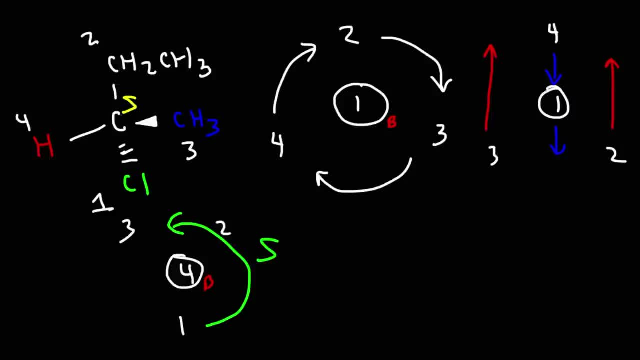 So that's the technique that you could use whenever group number four is not in the front or in the back. 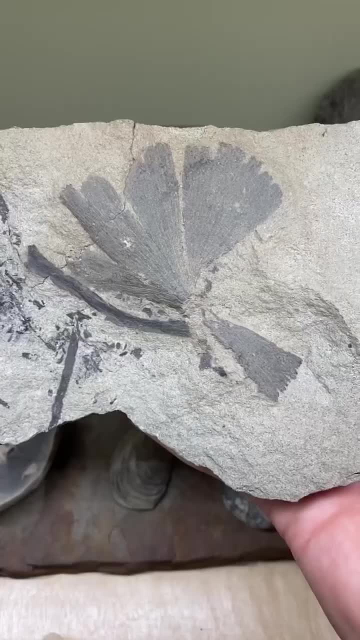 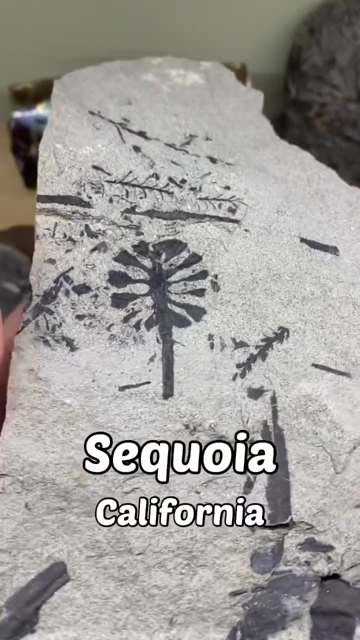 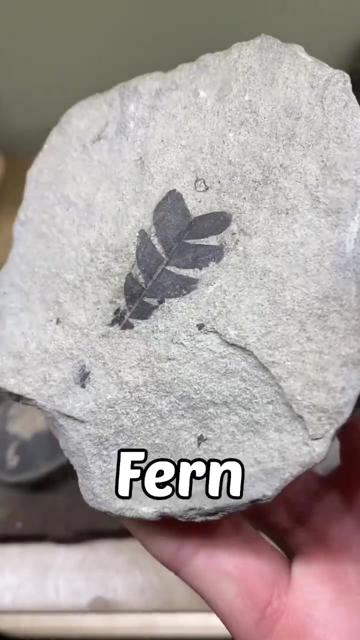 Many plants from the cretaceous period can still be found today, whether it be this ginkgo, which can still be found in asia, or this sequoia, which can be found in parts of california. and those that are not around today have modern relatives such as this pine and this fern fossil 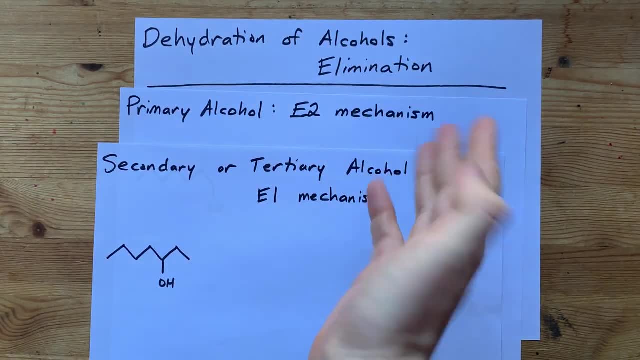 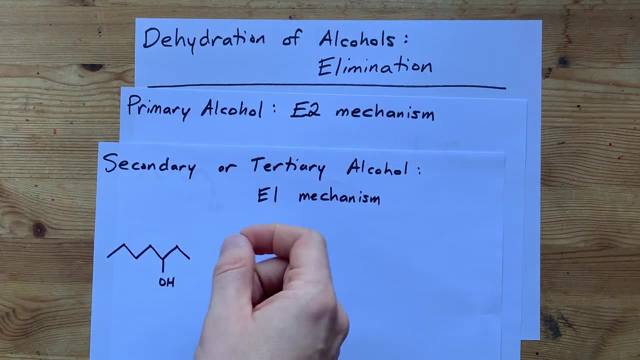 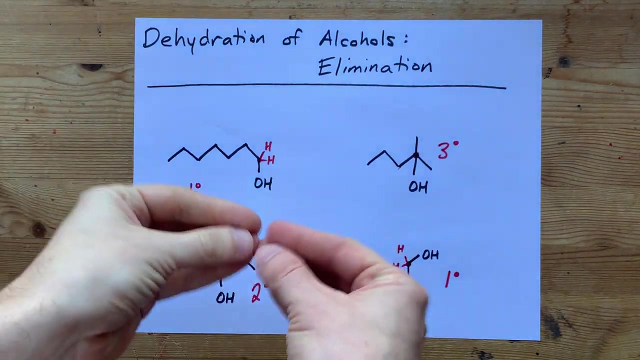 The dehydration of alcohols to create alkenes is an elimination reaction. The mechanism is going to depend on whether or not you start with a primary alcohol or a secondary or tertiary alcohol. So before you decide which one you're going to use, let's make sure we're all on the 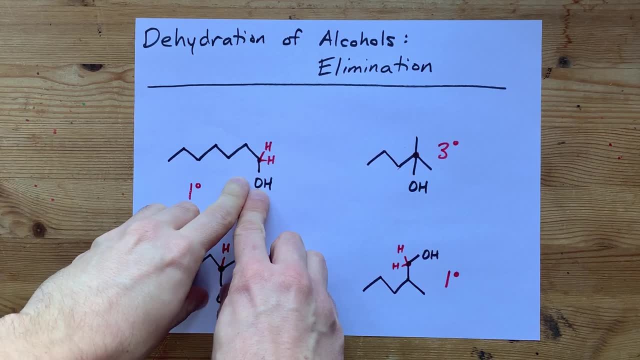 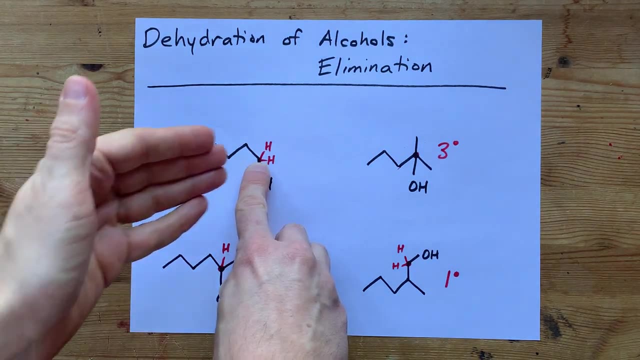 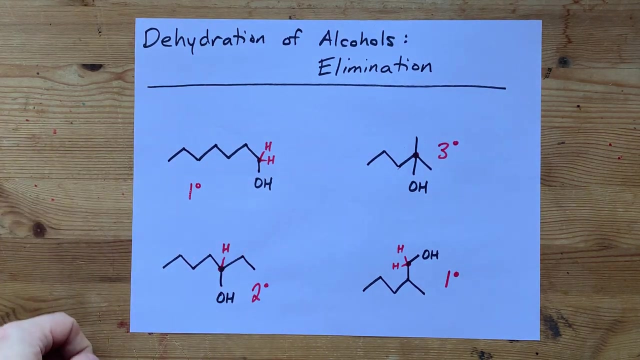 same page about what those words mean. This molecule, the OH, is connected to this carbon. They go through this related process and then nitrate, which is a LGB nelacансer, enters this攝dra. This is connected here, so that's another carbon. The question is: